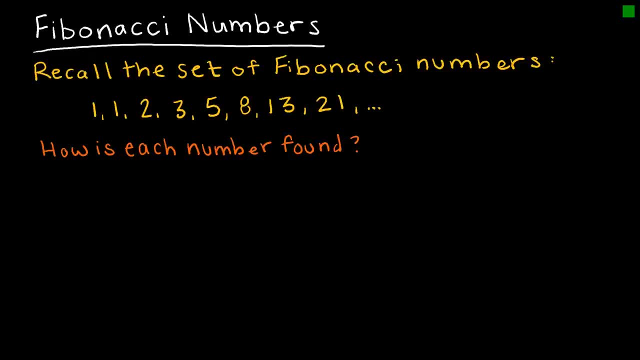 remember from back when you first learned about Fibonacci numbers. in order to find the next number, we just add the two items before, So to find, and we'll just say there's a pretend 0 here in front. so to find this value, I'm taking 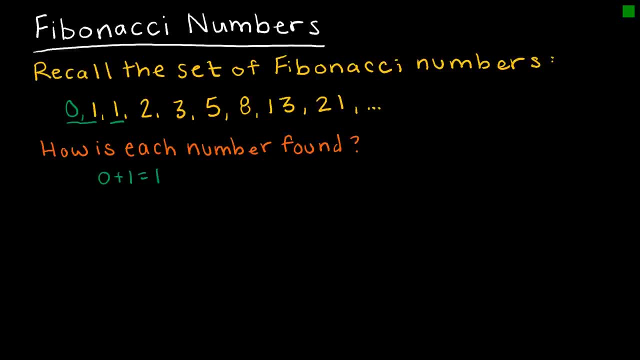 0 plus 1 to be equal to 1.. And then to find the value of 2, I'm taking 1 plus 1.. And then to find the value of 3, I'm taking 1 plus 2.. And we get the idea that 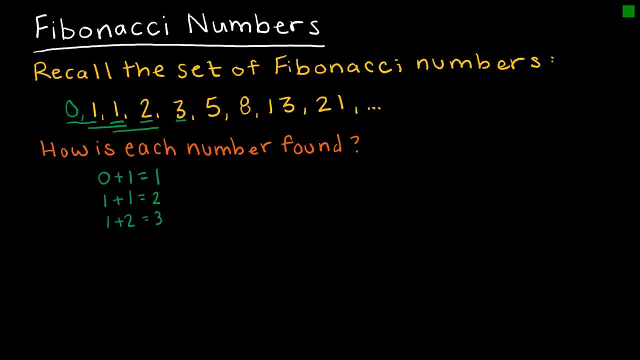 we would just continue this over and over and over. So this section we're going to be talking about recursive algorithms or recursive definitions, I guess, And what we would say here is, again in the non mathy way, we would say that we add the two numbers before and that would give us the next. 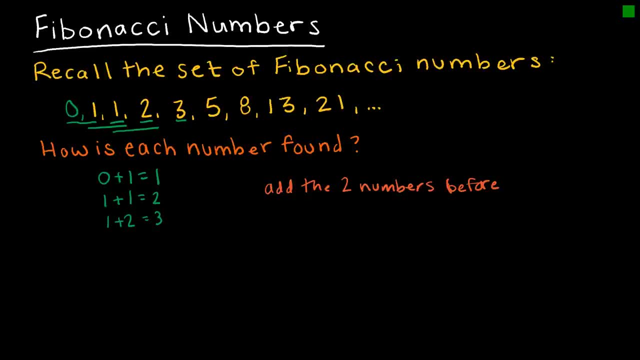 number. So again, that's the non mathy way to say it- We're just saying, hey, take the two numbers before and add them together. Now the problem with that is I need to know what the first two numbers are. So I really need to define that my imaginary first number would be 0 and that my real 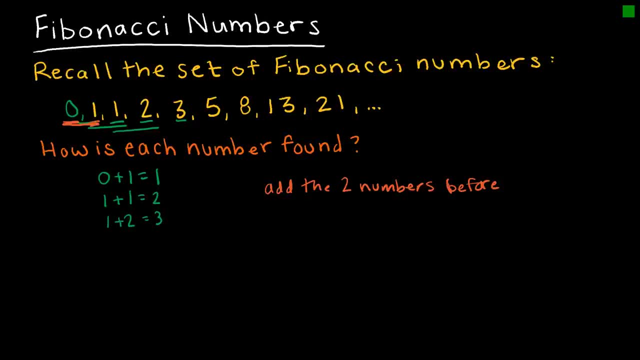 first number is 1.. And so this is how we would write this. We would say: let's let the very starting point be 0 and then let's let the first item in my set, which is that first initial point, when my second third, So we're going to write the second two numbers in here, And then I'm going to write 3 for the 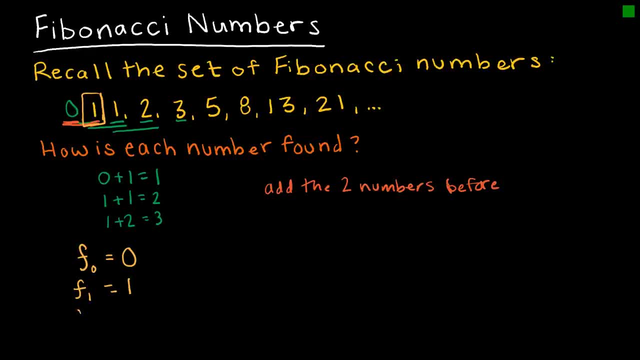 yellow number be 1.. And then let's let every other number be the number just before that, which we would say is f of n minus 1, so reduce that index by 1, and the number 2 before that. So this is how we would recursively define the Fibonacci numbers. So notice what we've done. 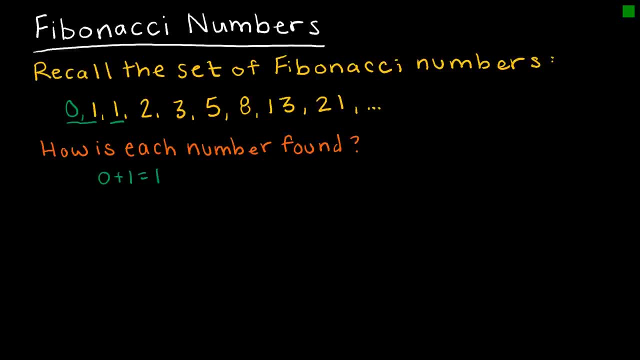 0 plus 1 to be equal to 1.. And then to find the value of 2, I'm taking 1 plus 1.. And then to find the value of 3, I'm taking 1 plus 2.. And we get the idea that 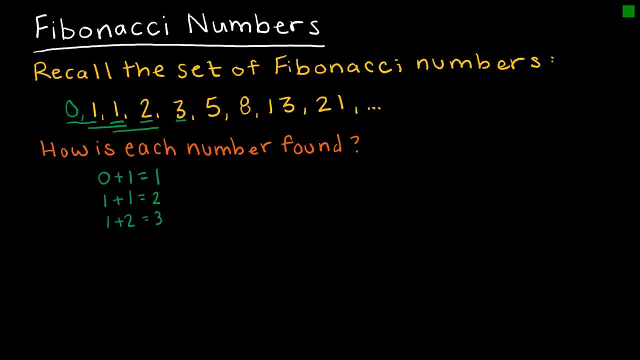 we would just continue this over and over and over. So this section we're going to be talking about recursive algorithms or recursive definitions, I guess, And what we would say here is, again in the non mathy way, we would say that we add the two numbers before and that would give us the next. 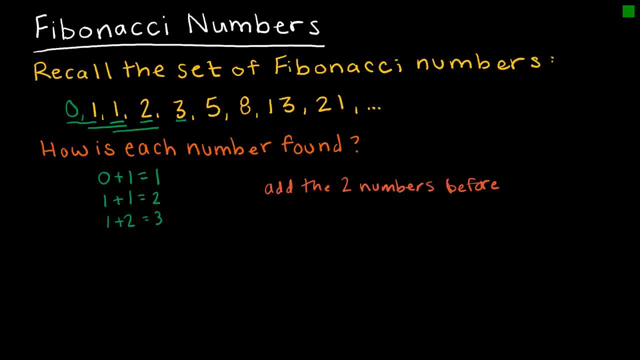 number. So again, that's the non mathy way to say it- We're just saying, hey, take the two numbers before and add them together. Now the problem with that is I need to know what the first two numbers are. So I really need to define that my imaginary first number would be 0 and that my real 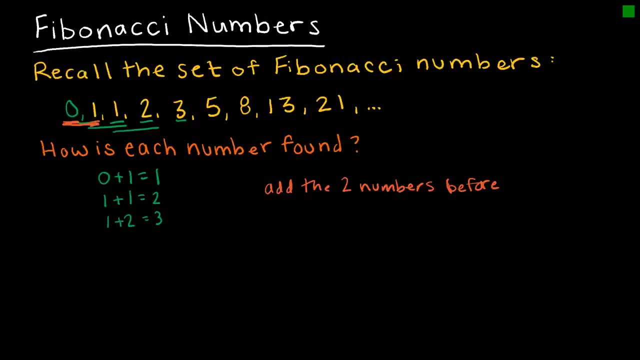 first number is 1.. And so this is how we would write this. We would say: let's let the very starting point be 0., And then let's let the first item in my set, which is that first yellow number, be 1.. And then let's let every other number be the number just before that. 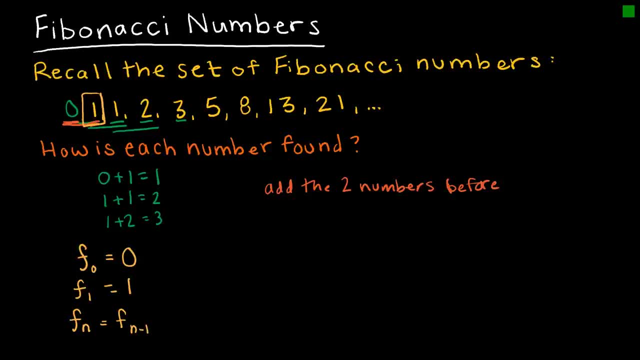 which we would say is f of n minus 1,. so reduce that index by 1, and the number 2 before that. So this is how we would recursively define the Fibonacci numbers. So notice, what we've done is we've looked at the sort of the starting point and the first value and in this case, 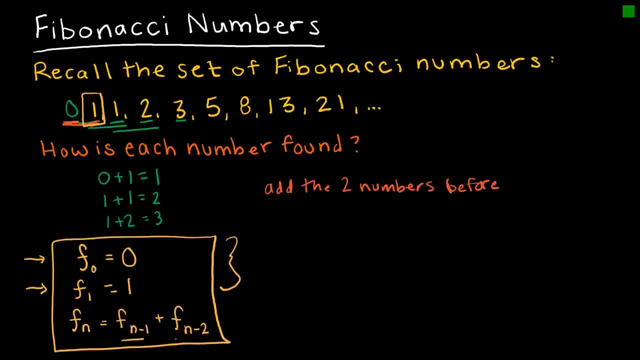 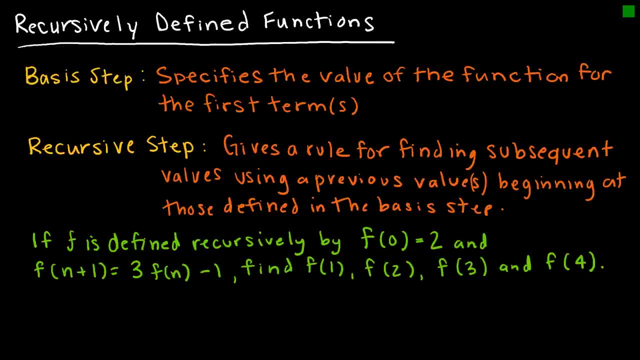 I had to define two values because I have to use two values in my recursive algorithm. So let's give it a formal definition. Recursively defined functions have a basis step and a recursive step. Now you might be thinking, hold on, this seems a lot like mathematical induction. 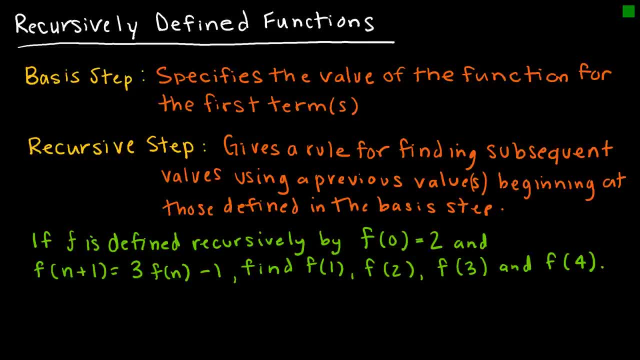 and you would be right. That's where we're going to be headed with this- is to be able to prove these using a form of mathematical induction. The basis step specifies the value of the function for the first term or terms. So in the one I just showed you, we specified two values. 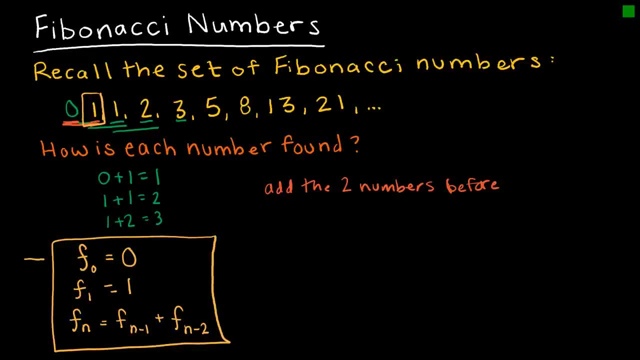 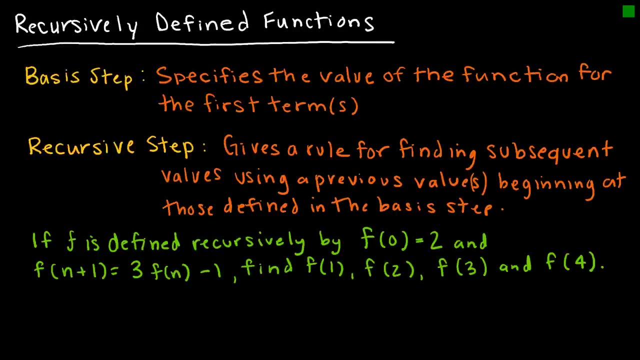 is, we've looked at the sort of the starting point and the first value and in this case I had to define two values because I have to use two values in my recursive algorithm. So let's give it a formal definition. Recursively defined functions have a basis step and a. 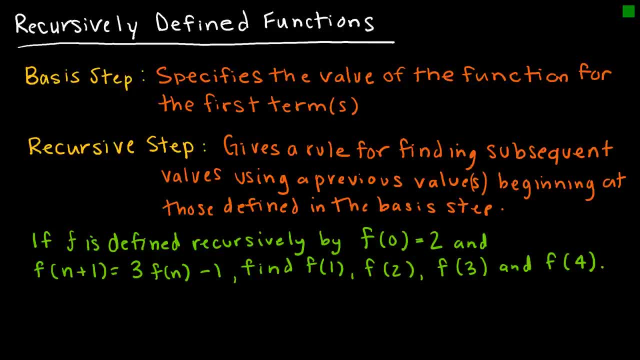 recursive step. Now you might be thinking: hold on, this seems a lot like mathematical induction, and you would be right. That's where we're going to be headed with this is to be able to prove these using a form of mathematical induction. 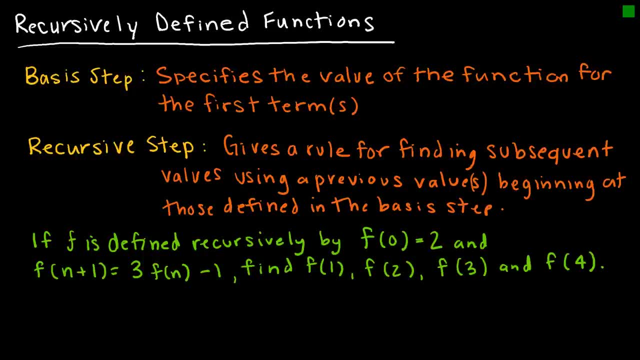 The basis step specifies the value of the function for the first term or terms. So in the one I just showed you, we specified two values, And the recursive step gives a rule for finding the subsequent values using a previous value or values, again starting at those that are defined in the basis step. So let's take a look at another. 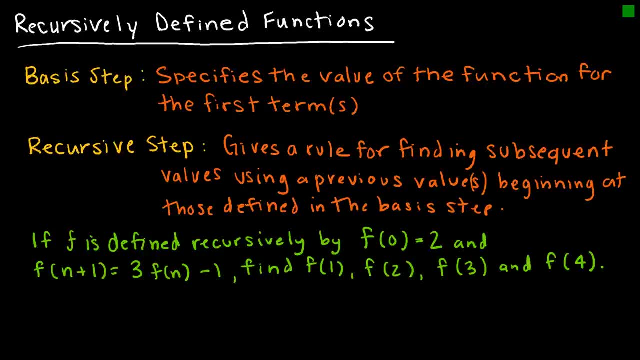 example, If F is defined recursively by F of 0 equals 2 and F of n plus 1 equals 3, Fn minus 1, they're asking me to find some values. So they're saying: okay, we're giving you sort of a starting point of 2.. If you wanted to give me the list, how would I find it? 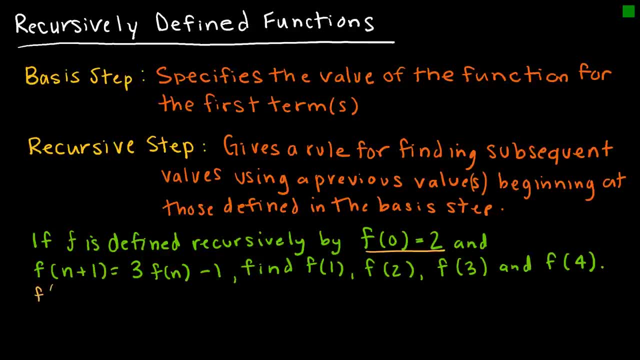 Well, if I want to find F of n plus 1, which I'm trying to find, F of 1, so that would be saying: let's take F of 0, plus 1. And that would be 3 times F of n, which means F of 0. So 3 times 2 minus 1,. 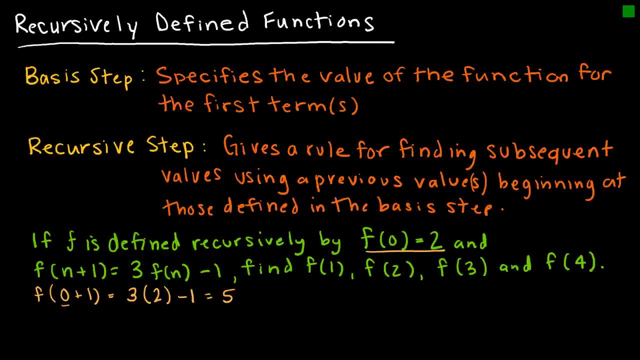 which is 6 minus 1, which is 5.. So F of 1 equals 5.. Then if I want to find F of 1 plus 1, which is of course F of 2, that would say take 3 times whatever you got before that. 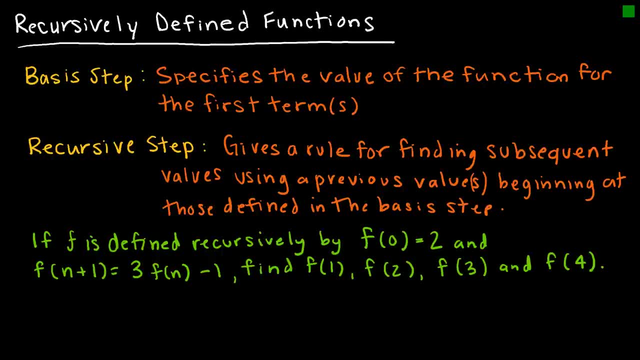 And the recursive step gives a rule for finding the subsequent values using a previous value or values, again starting at those that are defined in the basis step. So let's take a look at another example. If F is defined recursively by, F of 0 equals 2 and F of n plus 1 equals 3, Fn minus 1,. 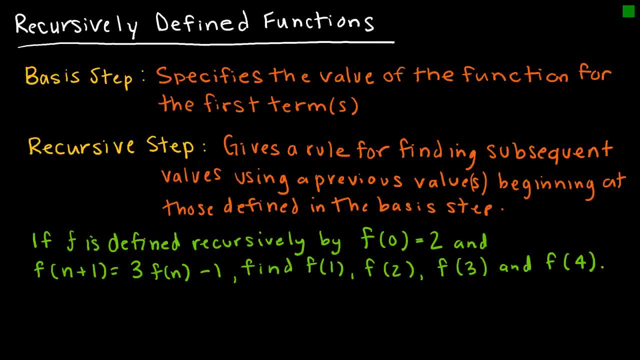 they're asking me to find some values, So they're saying: okay, we're giving you sort of a starting point of 2.. If you wanted to give me the list, how would I find it? Well, if I want to find F of n plus 1, which I'm trying to find, F of 1, so that would be. 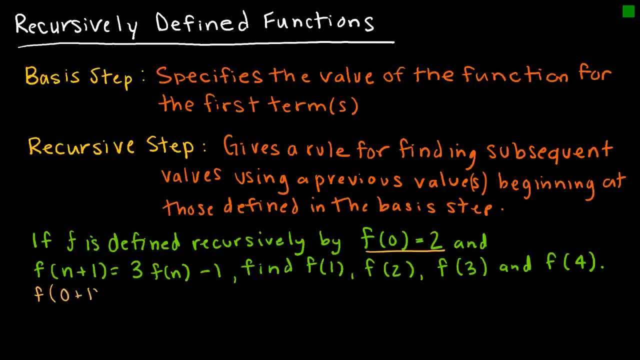 saying: let's take F of 0, plus 1. And that would be 3 times F of n, which means F of 0. So 3 times 2 minus 1,, which is 6 minus 1, which is 5.. So F of 1 equals 5.. Then if I want to find F of 1 plus 1,, 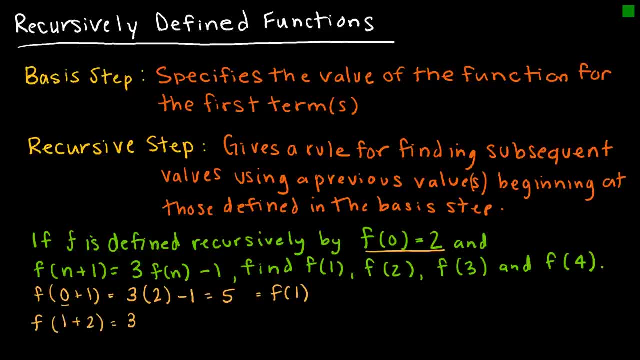 which is of course F of 2, that would say, take 3 times whatever you got before that, which is 5 minus 1.. So 15 minus 1 is 14, and that's F of 2.. And then again to find the next value. so if I said 2 plus 1 or F of 3, I would take: 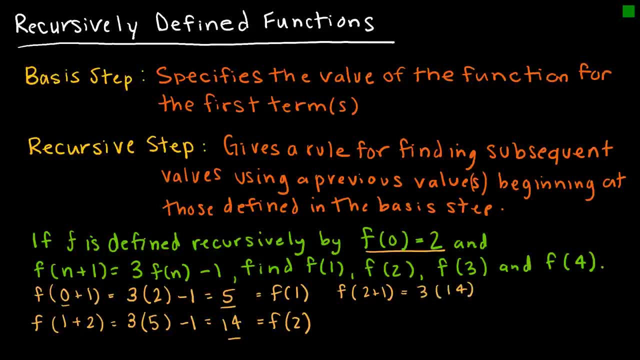 3 times 14 minus 1.. So that's 42 minus 1 or 41. That would be my value for F of 3.. And then if I wanted to find F of 4, remember that's just F of 3 plus 1.. So F of 4 is 3 times 41 minus 1.. 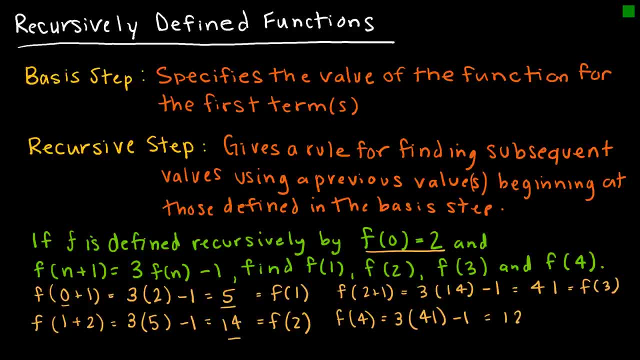 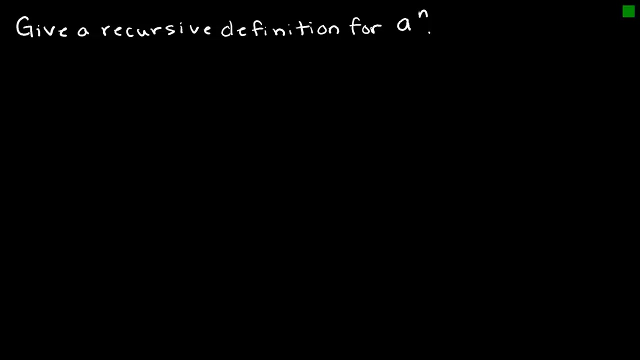 And 3 times 41 is 123 minus 1 is 122.. So I've used a recursive definition to find the first four items of this sequence and that would be 5, 14, 41, 122.. So let's see if we can come up with a recursive definition for A to the n. And let's assume A is. 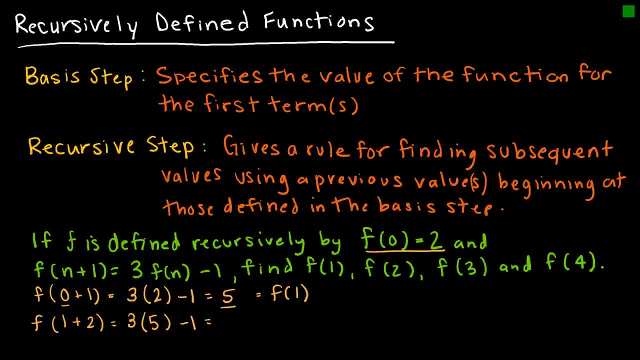 which is 5 minus 1.. So 15 minus 1 is 14.. And that's F of 2.. And then again to find the next value. So if I said 2 plus 1 or F of 3, I would take 3 times 14 minus 1.. So that's 42 minus 1 or 41. That would be my value for F of 3.. And then if I wanted to find F of 4,, 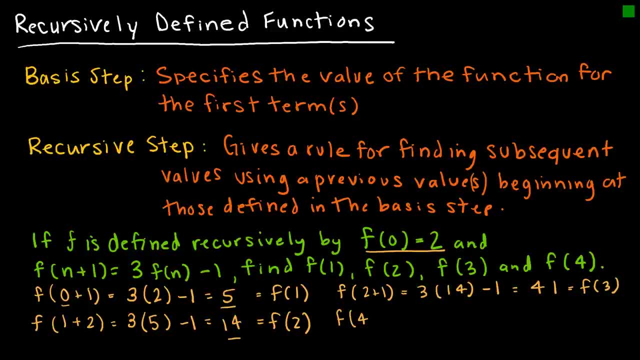 remember that's just F of 3 plus 1.. So F of 4 is 3 times 41 minus 1.. And 3 times 41 is 123 minus 1 is 122.. So I've used a recursive definition to find the first four items of this sequence, And that would be 5,, 14,, 41,. 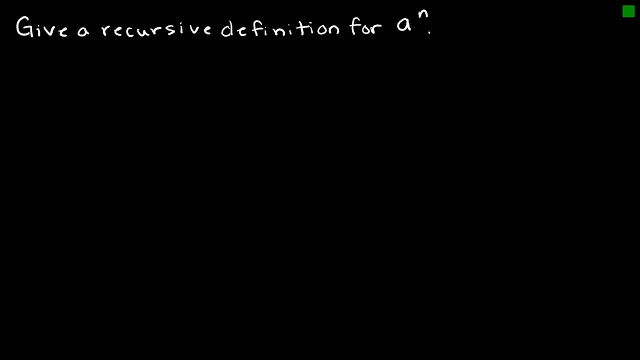 14,, 41,, 42,. So let's see if we can come up with a recursive definition for A to the end. And let's assume A is nonzero real And let's assume N is a non negative integer. So what we're saying is we know how to find A to the end. 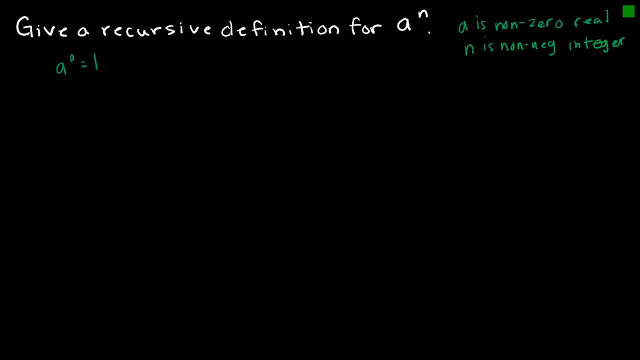 If you had a to the 0, it would be 1.. a to the 1 would just be 1a right. a to the 2 would be a times a. We get the idea. So what we want to do is we want to create an algorithm. 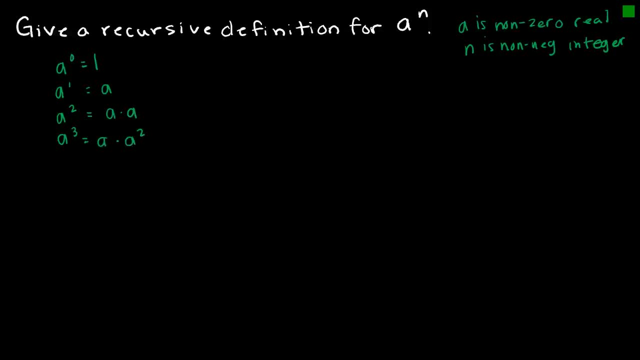 that helps us to determine exactly how we could find the next value based on the value before. And so you see, I've started to build a little bit of a pattern. If I had a to the 5th, I would really just be taking a times a to the 4th, etc. 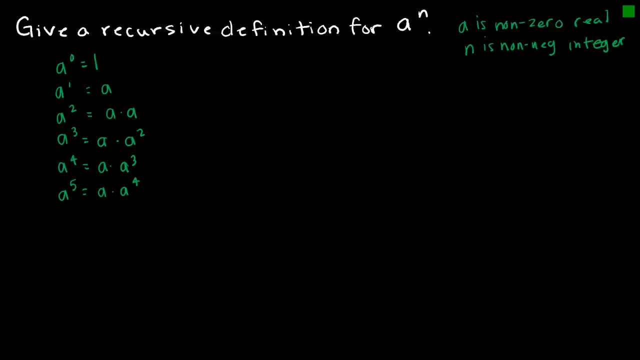 So, remember, in order to have a recursive definition, we have to define the basis, which means we have to define it at the lowest level. And so we're going to say a of 0 is equal to 1.. Because, anyway, The only thing to the 0 power is 1.. 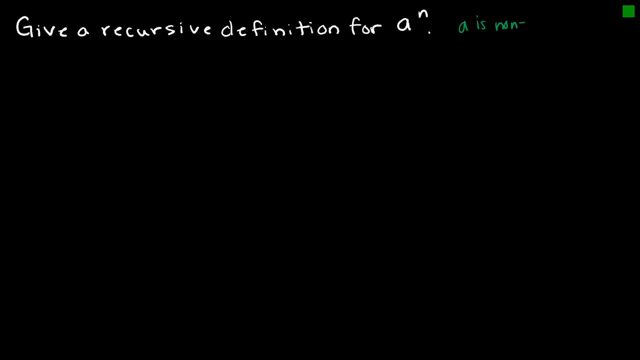 non-zero real And let's assume n is a non-negative integer. So what we're saying is: we know how to find A to the n, So let's assume A is non-zero real And let's assume n is a non-negative integer. 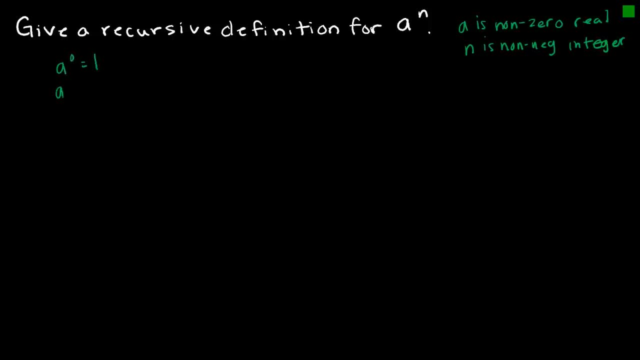 If you had A to the zero, it would be 1.. A to the one would just be 1A right. A to the two would be A times A. we get the idea. So what we want to do is what we want: to create an algorithm. 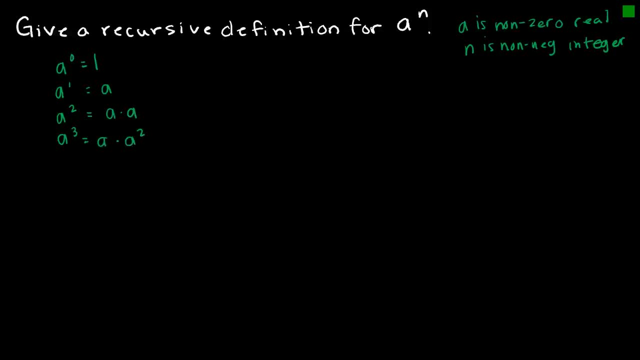 that helps us to determine exactly how we could find the next value based on the value before. And so you see, I've started to build a little bit of a pattern. if I had A to the fifth, I would really just be taking A times A to the fourth, etc. 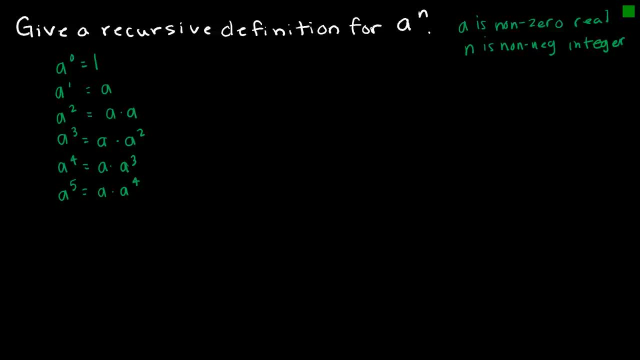 So, remember, in order to have a recursive definition, we have to define the basis, which means we have to define it at the lowest level. And so we're going to say A of zero is equal to one, because any of those values would be equal to one. 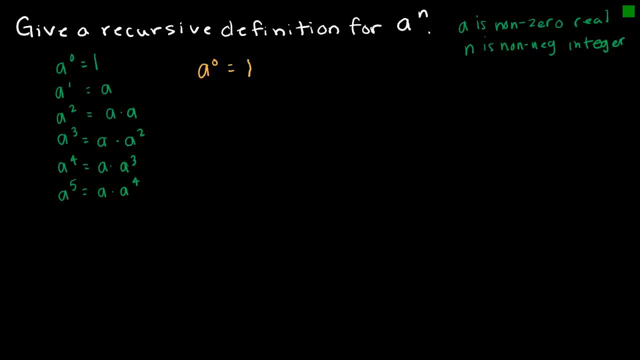 to the zero power is 1. so that's the sort of the basis step. then the recursive step says: how do I find a to the n plus 1? so to find the next value up, essentially what I'm going to do, and again looking at my little pattern over: 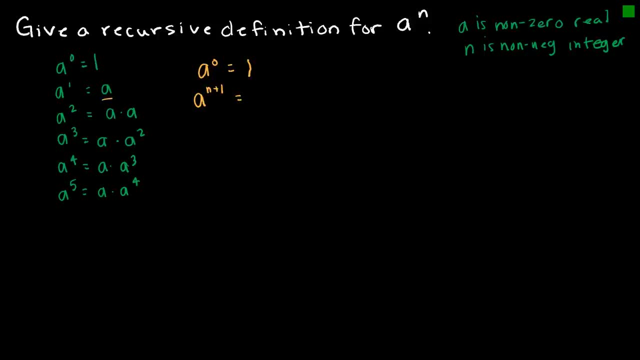 here I'm saying: okay, to find a squared, I took a times a and to find a to the third, I took a squared times a. so notice, I'm just taking one value before and taking it times a, which means I can write that as a times a to the n, because 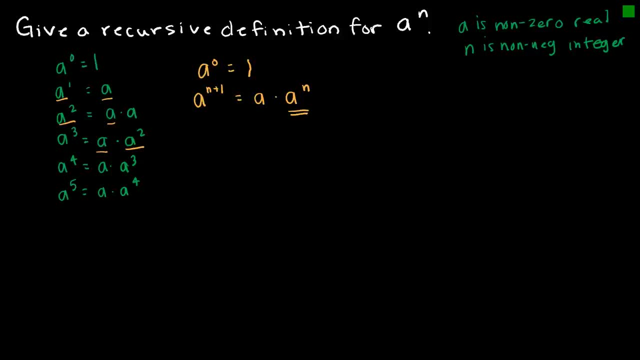 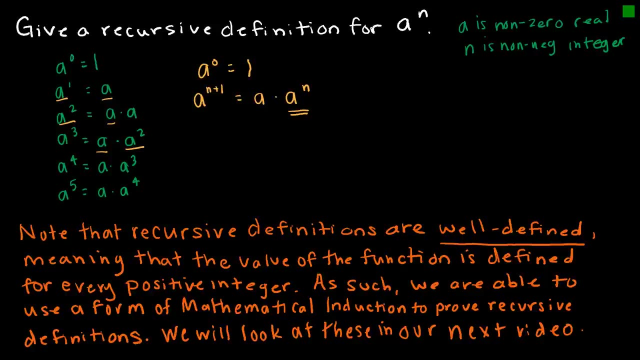 I'm taking whatever the value was before that and I'm multiplying it again by a. so notice that these are going to be considered well-defined, and well-defined just means that the value of the function is defined for every positive integer, and the reason that's important is that 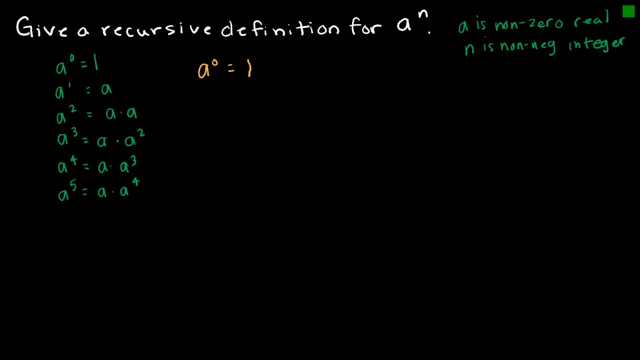 So that's sort of the basis step. Then the recursive step says: how do I find a to the n plus 1?? So to find the next value up, essentially what I'm going to do. And again, looking at my little pattern over here, I'm saying: 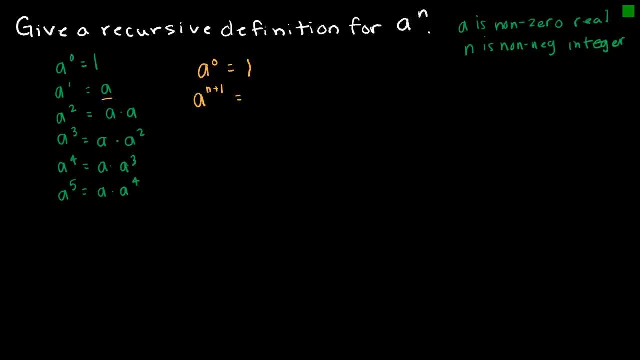 okay, to find a squared, I took a times a, And to find a to the 3rd, I took a squared times a. So notice, I'm just taking one value before and taking it times a, Which means I can write that as a times a to the n. 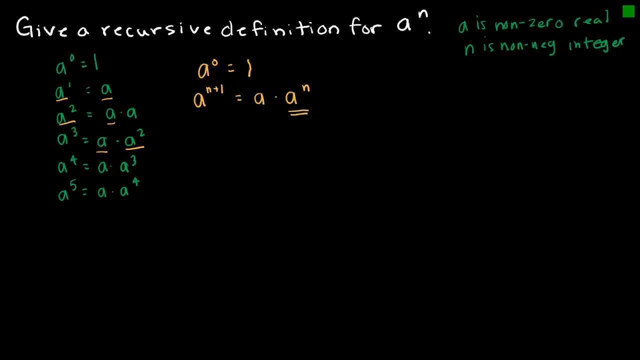 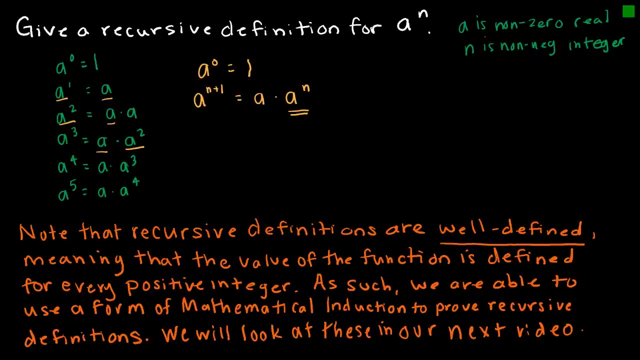 Because I'm taking whatever the value was before that and I'm multiplying it again by a. So notice that these are going to be considered well-defined, And well-defined just means that the value of the function is defined for every positive integer, And the reason that's important is that allows us to use mathematical induction. 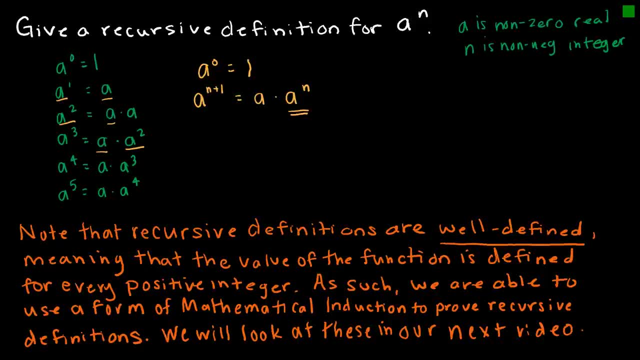 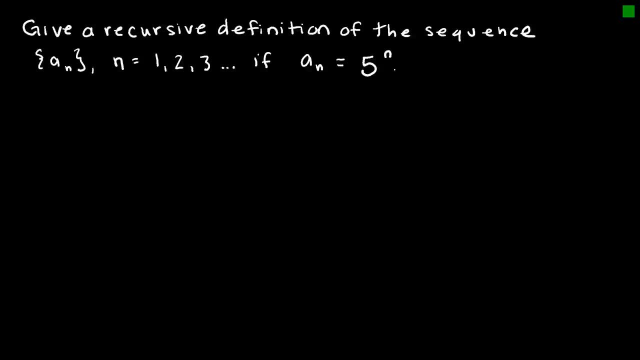 or, in this case, a form of mathematical induction to prove recursive definitions, which we'll look at in our next video. So let's give a recursive definition for the sequence a sub n where n is 1,, 2,, 3,, etc. if a sub n is equal to 5n. 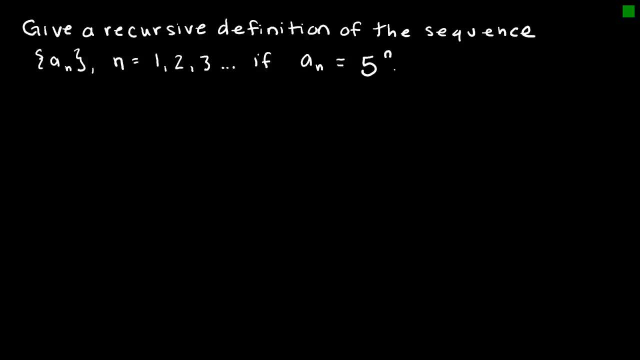 So again, we already know how to find each value of the sequence, and it's not a bad practice if you, If it doesn't come to you right away how to write this recursively. it's not a bad practice to give yourself some leeway in finding some of those first values. 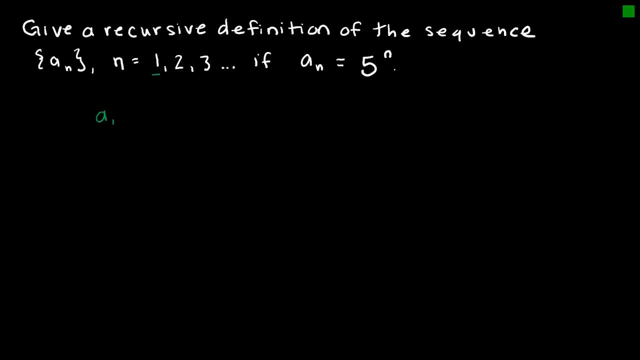 So remember we're starting with 1.. So if I had a1, that would be 5 to the 1,, which is just 5.. And then a2 would be 5 squared, which is the same as 5 times 5.. 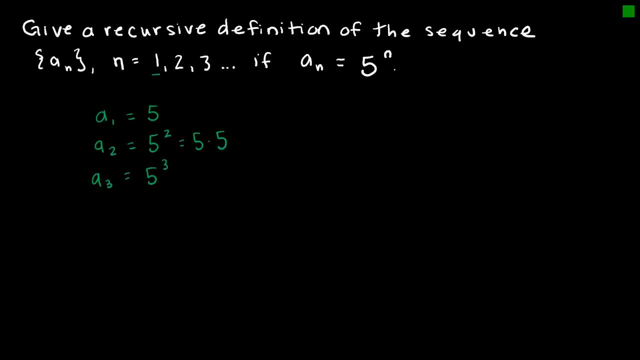 And a3 is equal to 5 cubed a4 is equal to 5 to the 4th. And how is this helping me? Because, remember, 5 to the 3rd is the same as 5 squared times 5.. 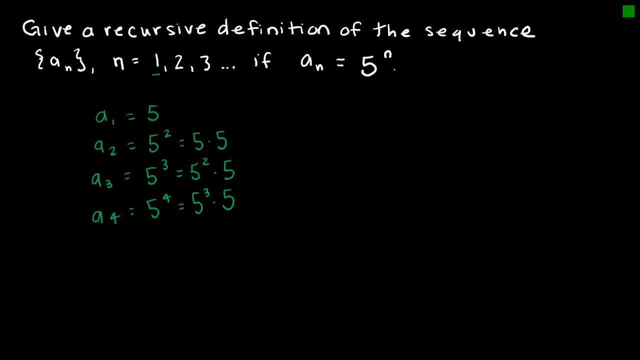 And 5 to the 4th is the same as 5 to the 3rd times 5.. And so you can see I'm sort of building a pattern. a2 was 5 squared, and if I take a2 times 5, I get a3.. 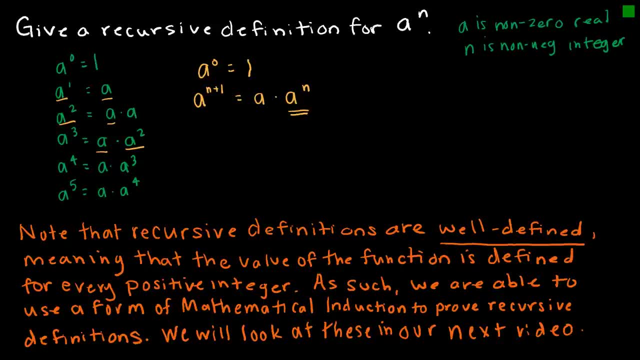 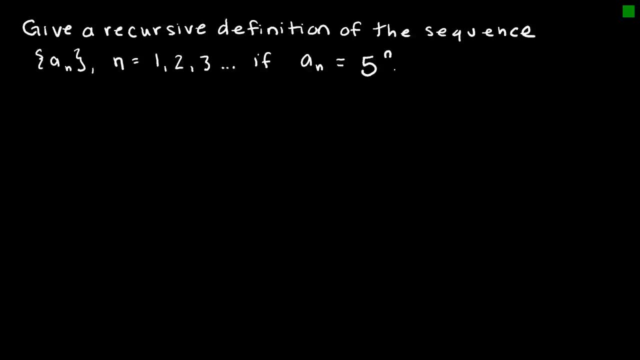 allows us to use mathematical induction, or in this case a form of mathematical induction, to prove recursive definitions, which we'll look at in our next video. so let's give a recursive definition for the sequence a sub n where n is 1, 2, 3, etc. if a sub n is equal to 5 n. so again, we already know how to find each value. 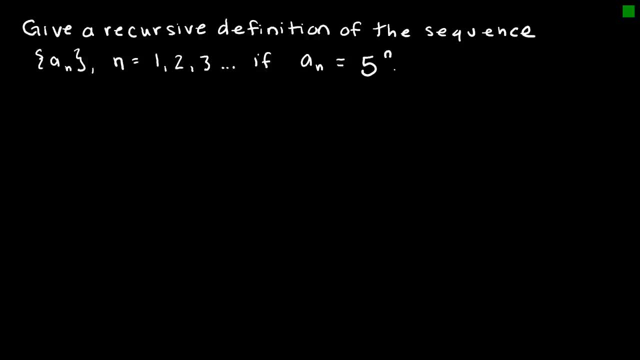 of the sequence, and it's not just the value of the sequence, it's the value of the element. if it's equal to 5, n and 2, 3, etc. that might be which layer the oxidation is the case. and that would be if everything on each of them is equal. 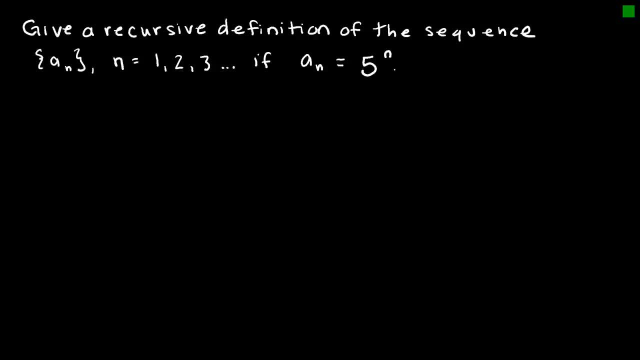 to a sub n plus a, some kind of minimum or a lower siguemum, and it is an 셨�равля a nerede a. if b is equal to b b, then we are left with a small reason when, if we take a proposal- for it's a very simple way to use PLAN- 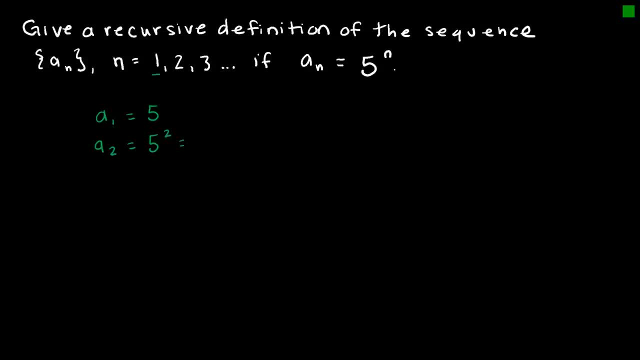 B, where n says 6, please, t is equal to 0, and a, which is double from 1, n and 2, which means a. show you right now. I don't have to go a little bit deep into everything, because the Claus polynomial is quite easy to draw up, so you don't have to. 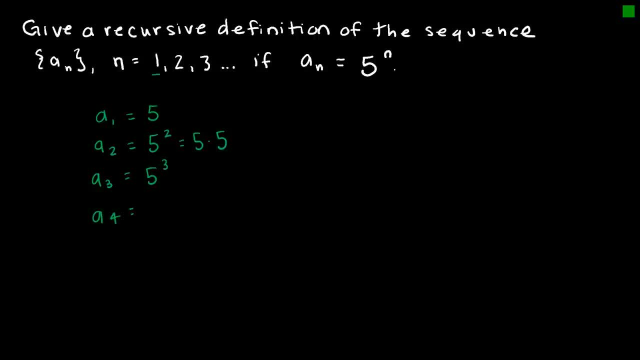 equal to 5 cubed, and a4 is equal to 5 to the fourth. And how is this helping me? Because, remember, 5 to the third is the same as 5 squared times 5, and 5 to the fourth is the same as 5 to. 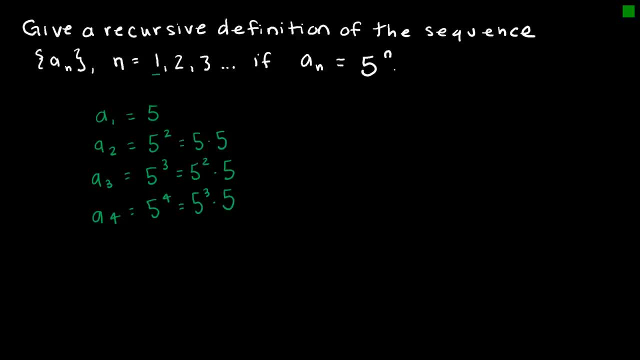 the third times 5.. And so you can see I'm sort of building a pattern. a2 was 5 squared, and if I take a2 times 5, I get a3.. And a3 was 5 cubed, and if I take 5 cubed times 5, I get a4.. So I've 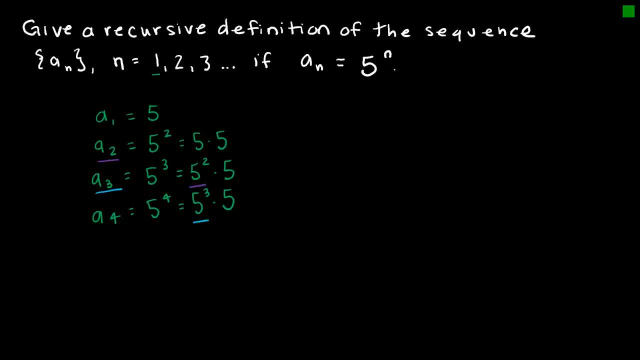 really already built my algorithm. I just have to now define it. Remember when we define it: we start by defining the first term in the sequence. So I'm going to define a sub 1 to be 5, and then every other value to find the next value in a sequence. I'm going to take a2 times 5, and if I take a3 times 5, I get a3.. And if I take a3 times 5, I get a3.. And I'm going to take a3 times 5, and if I take a3 times 5,, I get a3.. And if I take a3 times 5, I get a3.. And 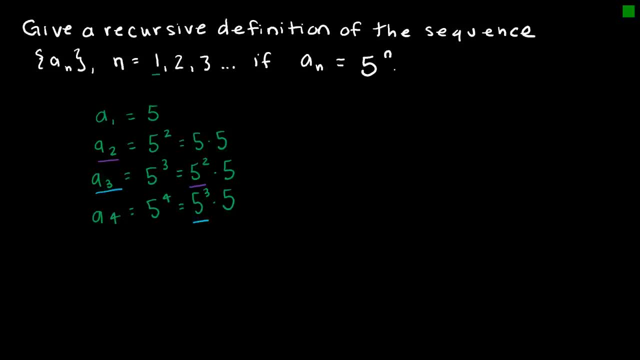 And a3 was 5 cubed, and if I take 5 cubed times 5, I get a4. So I've really already. I've already built my algorithm. I just have to now define it. Remember, when we define it, we start by defining the first term in the sequence. 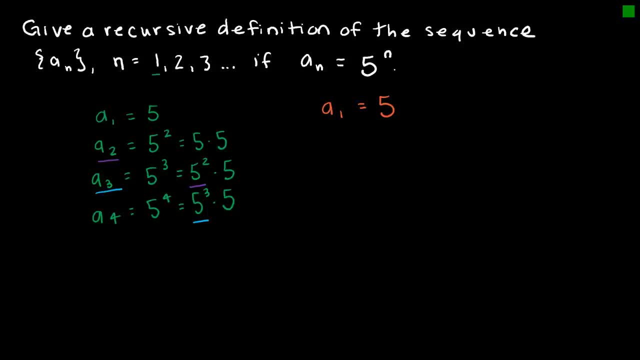 So I'm going to define a sub 1 to be 5.. And then every other value to find the next value in a sequence. I'm going to take 5 times whatever the value was before for n that is greater than 1.. 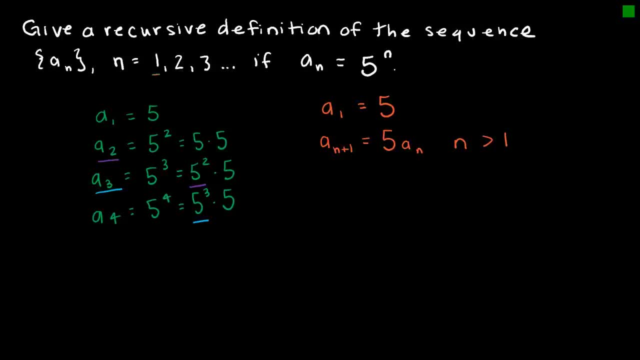 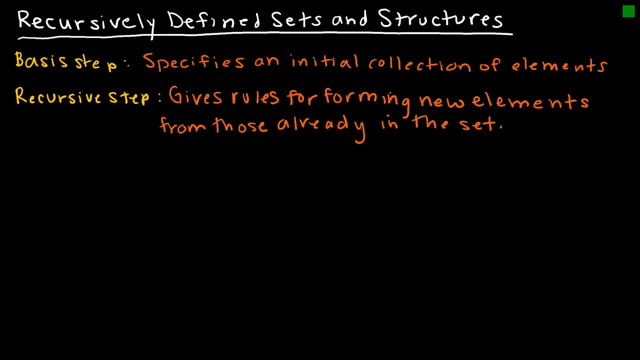 So greater than 1, because it already told me: Sorry, greater than or equal to 1, because it's telling me 1 here And then now for everything greater than or equal to that. that's how I find the next value. So we just looked at recursive functions. 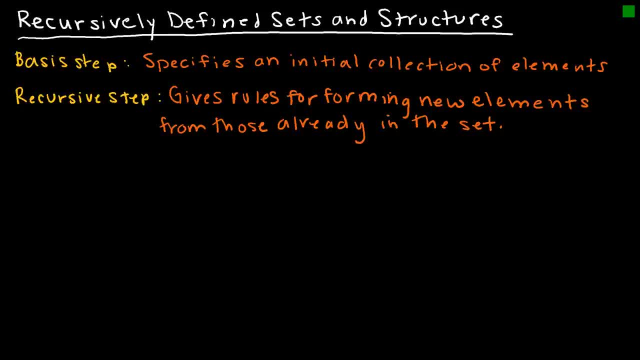 Now I want to look at recursively defined sets and structures And again I want you to notice, the basis step specifies the initial collection of elements. So in this case, it might be a set of elements. So in this case, it might be a set of elements. 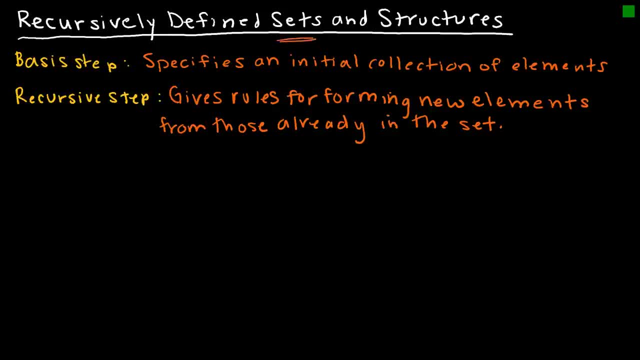 be a set of elements, which is why, of course, we're looking at sets and structures. so it specifies what the initial collection of elements is. the recursive definition gives the rules for forming new elements from those already in the set, so it's really exactly what we did for functions. this is: 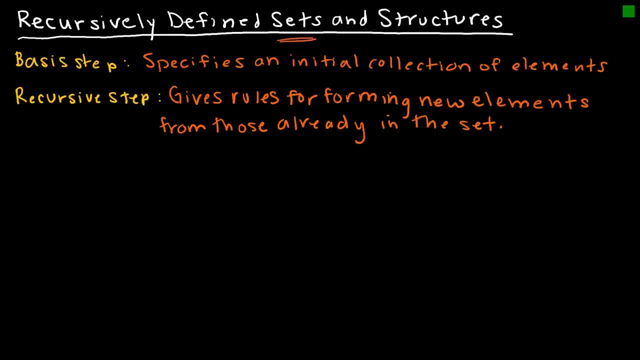 just specific to sets. so, for example, let's say we want a recursive definition for the natural numbers which, remember, the natural numbers are the counting numbers, um, starting at zero, basically. so zero one, two, et cetera, et cetera, et cetera. so the pace, the basis step, would say: 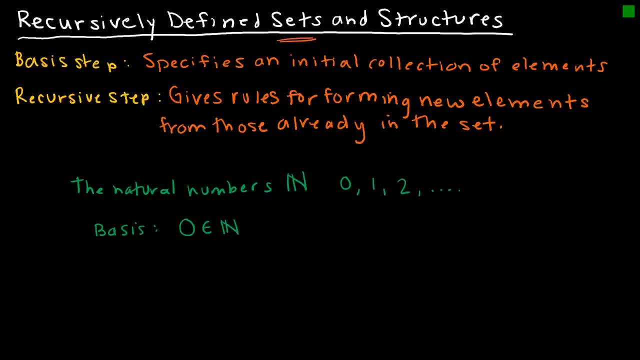 that zero belongs to the natural numbers and that's saying that is my initial collection is zero. the recursive step says how am i going to find, starting with zero, all of the other numbers? so i can say if n is an element of the natural numbers, then n plus 1 is an element of the natural numbers. 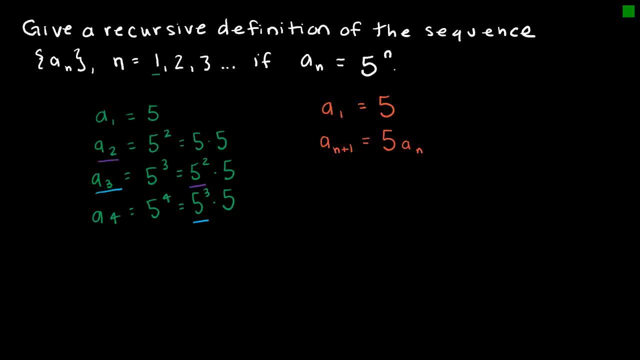 I'm going to take a3 times 5, and if I take a3 times 5, I get a3.. And I'm going to take 5 times whatever the value was before for n, that is greater than 1.. So greater than 1, because it. 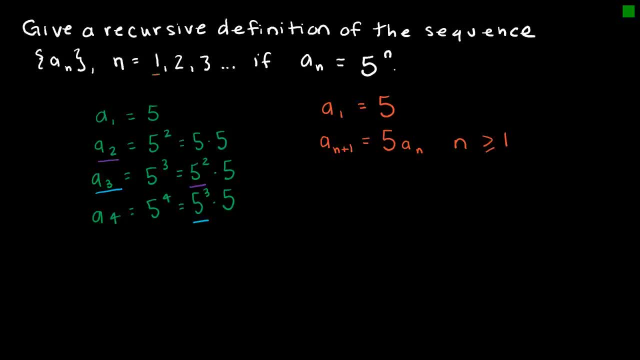 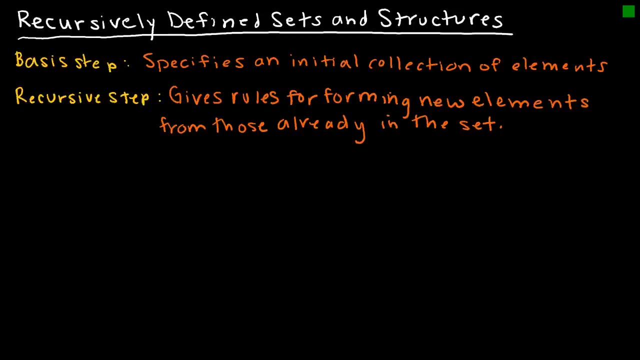 already told me, sorry, greater than or equal to 1, because it's telling me 1 here and then now for everything greater than or equal to that. that's how I find the next value. So we just looked at recursive functions. Now I want to look at recursively defined. 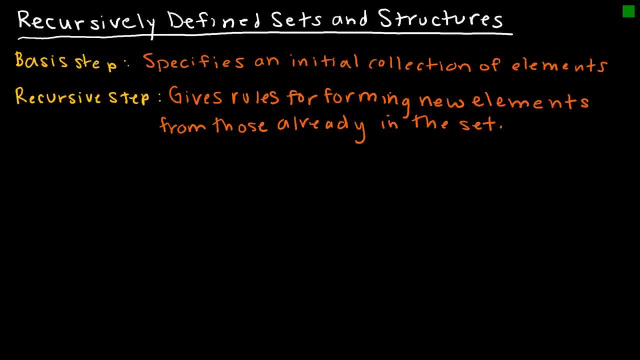 sets and structures. And again I want you to notice, the basis step specifies the initial collection of elements. So in this case it might be a set of elements, which is why, of course, we're looking at sets and structures. So it specifies what: the initial collection of elements. 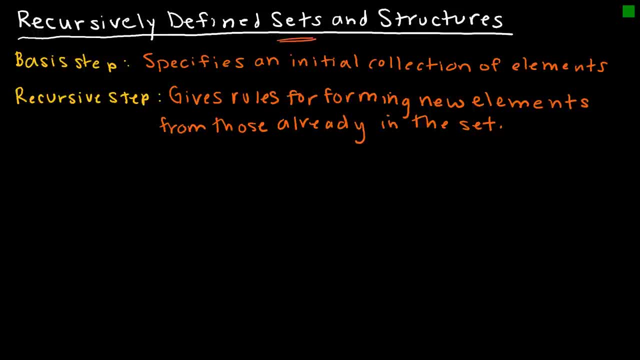 is, The recursive definition gives the rules for forming new elements from those already in the set. So it's really exactly what we did for functions. This is just specific to sets. So, for example, let's say we want a recursive definition for the natural numbers. 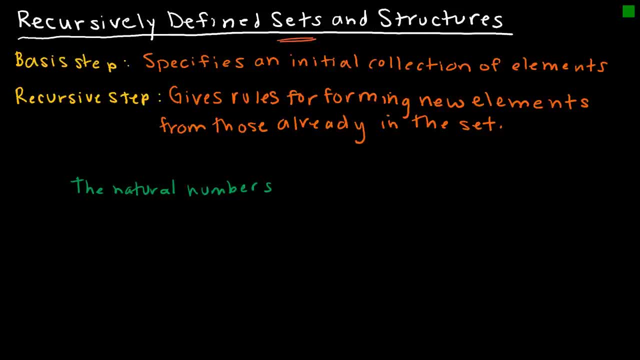 which, remember, the natural numbers are the counting numbers starting at zero, basically. So zero, one, two, et cetera, et cetera, et cetera. So the page, the basis step, would say that zero belongs to the natural numbers, And that's saying that is my initial collection. 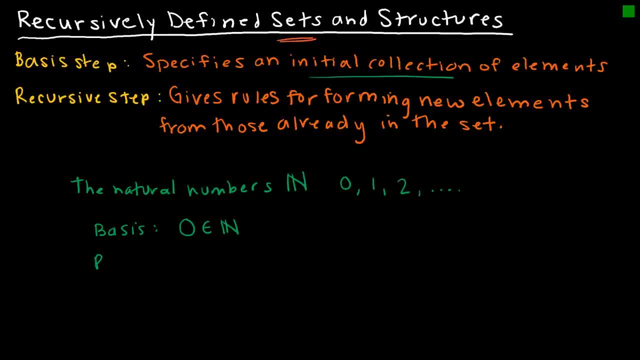 is zero. The recursive step says: how am I going to find, starting with zero, all of the other numbers? So I can say: if n is an element of the natural numbers, then n plus one is an element of the natural numbers, Just like that. So again I'm starting. 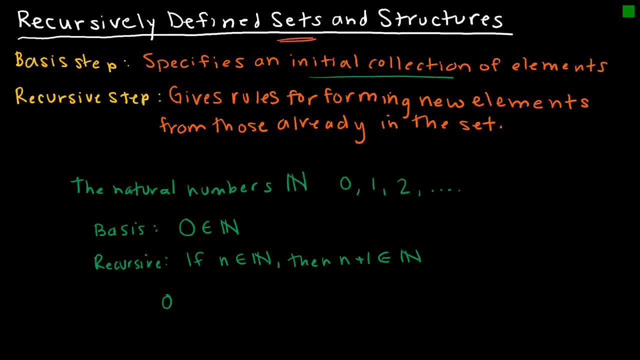 with zero. And then the recursive part would say: hey, zero is in the natural numbers, therefore n plus one or one is in the natural numbers. And then it says: hey, one is in the natural numbers, then n plus one or two is in the natural numbers. 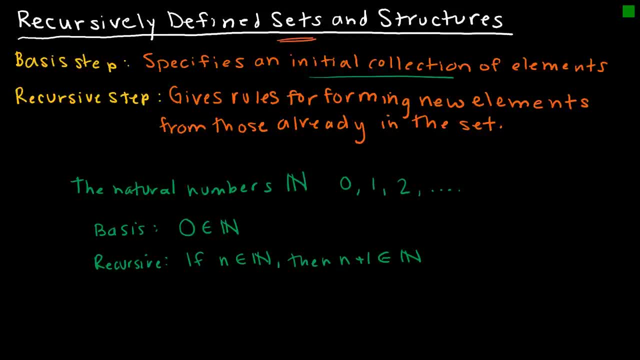 just like that. so again, i'm starting with zero, and then the recursive part would say: hey, zero is in the natural numbers, therefore n plus 1 or 1 is in the natural numbers. and then it says: hey, 1 is in the natural numbers, then n plus 1. 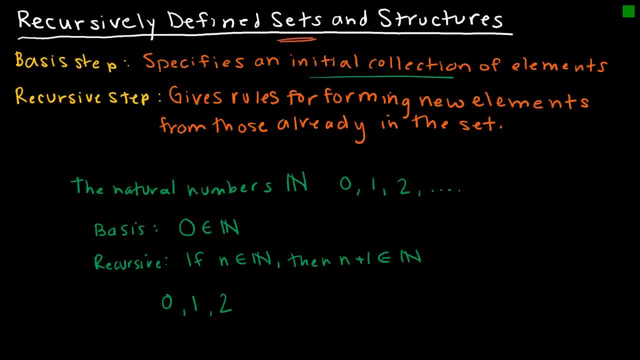 or 2 is in the natural numbers. and since 2 is in the natural numbers, then n plus 1, which is 2 plus 1 or 3, is in the natural numbers, and we can see how that would continue. so let's look at another. 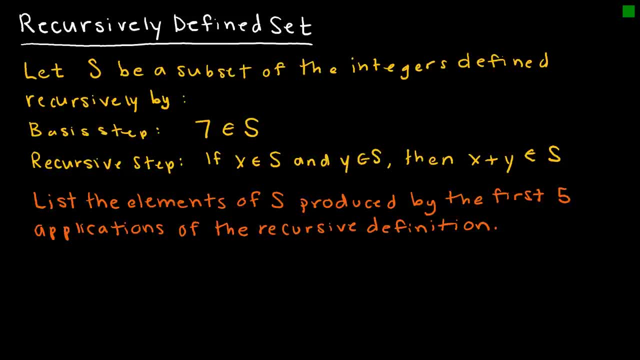 recursively defined set and that set says: s is a subset of the integers defined recursively by the basis step that 7 is an element of s and the recursive step that if x is an element of s and y is an element of s, then their sum is also an element of s. so if we wanted to use that to, 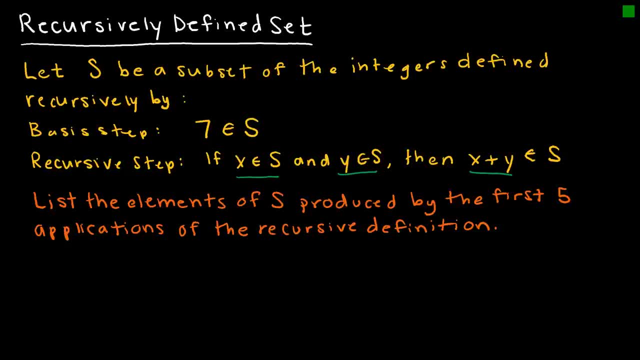 list the elements of s produced by the first five applications of the definition. the first value would be 3.. 7 because the first value comes from the basis step. so i've applied it once. applying it a second time gives me the first recursive step, which is: 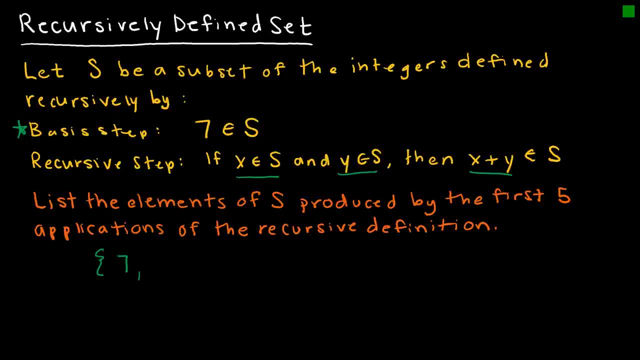 if x is an s and y is an s, then x plus y is an s, and so essentially that's saying 7 is an s and also 7 is an s, and so the sum of 7 and 7, which is 14, is an s. so that's really step 2, because step 1 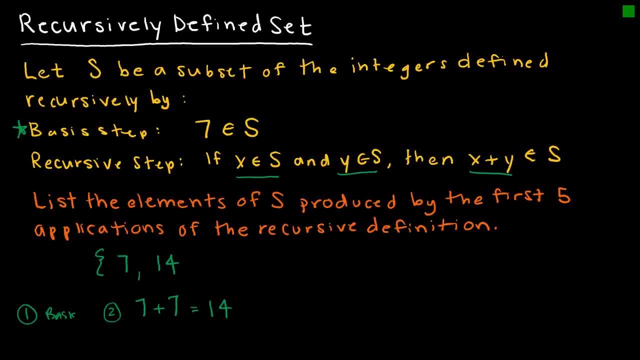 was the basis step that said 7 is in there. then step 3 says if x is in s and y is an s, then the sum of those is in s, which is 21, and you can see this process. if i'm doing it five times, i would then take 7 plus 21 and that's 28. 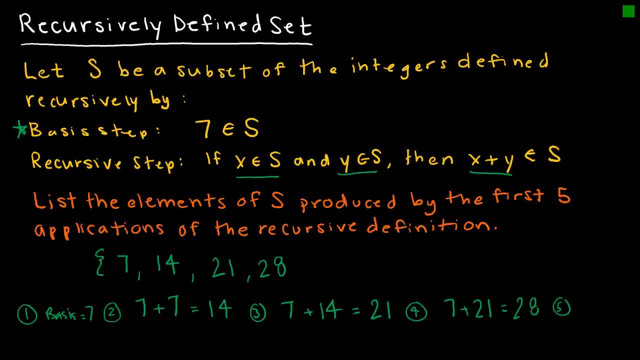 and then 28 plus 21 plus 7, and that is 35. now you might be asking then: well, why wouldn't I add 14 and 35 together? why couldn't that be a step? and it certainly could be a step. I just wanted to get the first five applications, which is essentially that. 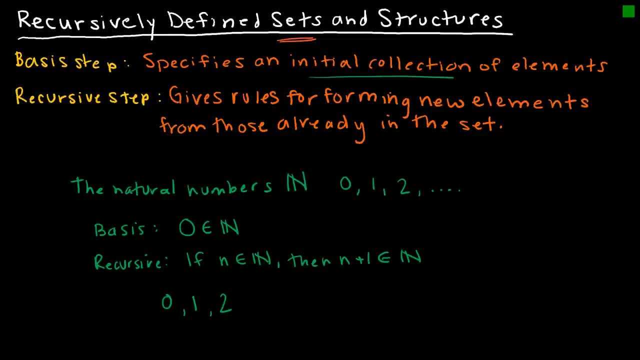 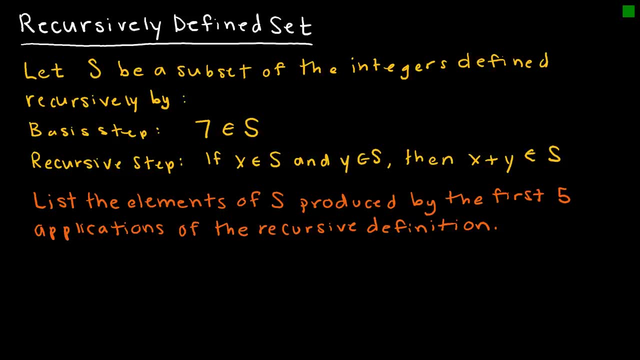 And that means zero is in the natural numbers. And since two is in the natural number, then n plus one, which is two plus one or three, is in the natural numbers, and we can see how that would continue. So let's look at another recursively. 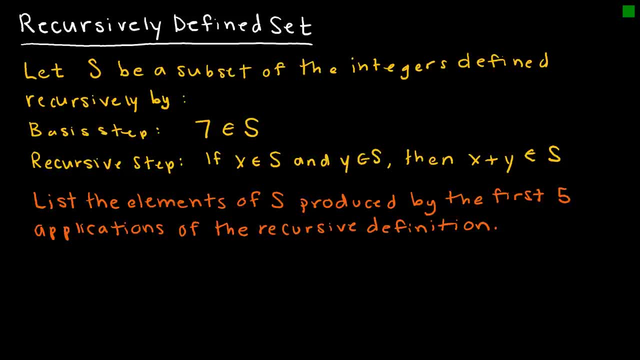 defined set And that set says S is a subset of the integers defined recursively by the basis step. that seven is an element of S And the recursive step, that is X is an element of S and y is an element of S, then their sum. 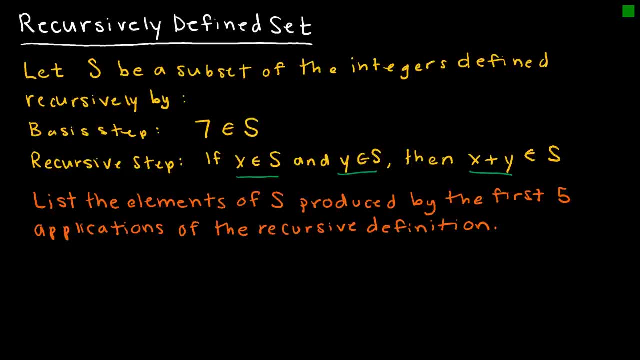 also an element of s. So if we wanted to use that to list the elements of s produced by the first five applications of the definition, the first value would be 7, because the first value comes from the basis step. So I've applied it once. 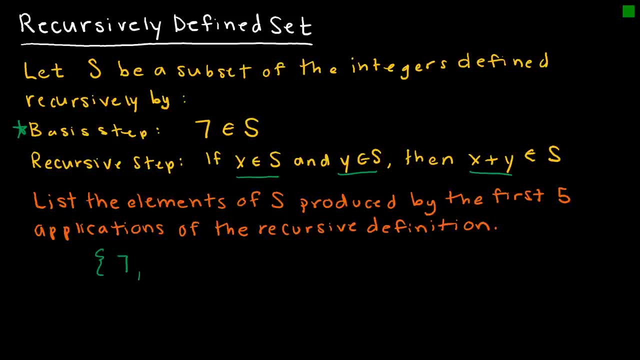 Applying it a second time gives me the first recursive step, which is: if x is an s and y is an s, then x plus y is an s, And so essentially, that's saying 7 is an s and also 7 is an s, And so the sum of 7 and 7, which is 14, is an s. So that's. 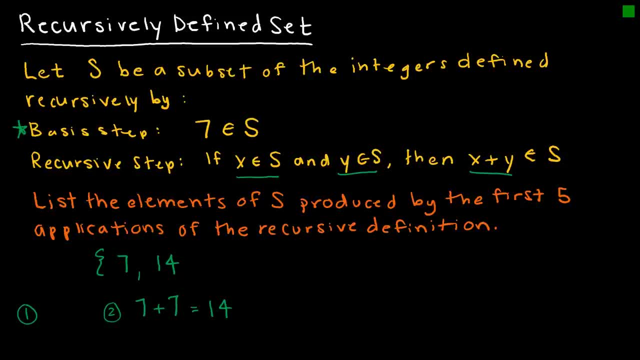 really step two, because step one was the basis step that said 7 is in there. Then step three says if x is in s and y is in s, then the sum of those is in S, which is 21.. And you can see this process if I'm doing it five times. 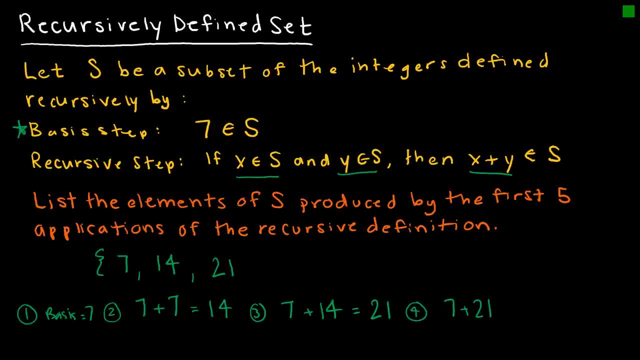 I would then take 7 plus 21,, and that's 28,, and then 28 plus 7,, and that is 35. Now you might be asking then: well, why wouldn't I add 14 and 35 together? 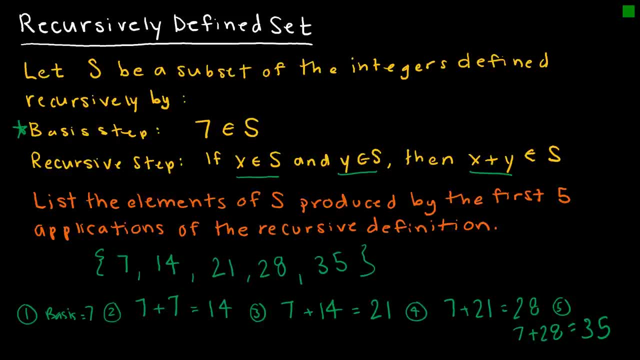 Why couldn't that be a step? And it certainly could be a step. I just wanted to get the first five applications, which is essentially that I'm adding 7 each time And notice, if I took 14 plus 35, that number which is 49,. 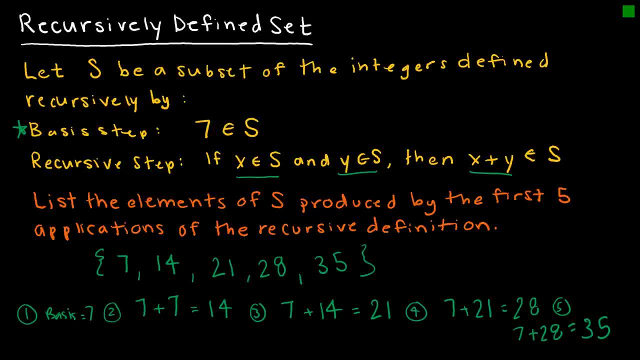 I'm adding seven each time and notice, if I took 14 plus 35, that number, which is 49, would in fact be what I would get if I took 42, which is what the next value would be plus 7. so I can add two other elements of the set together and that. 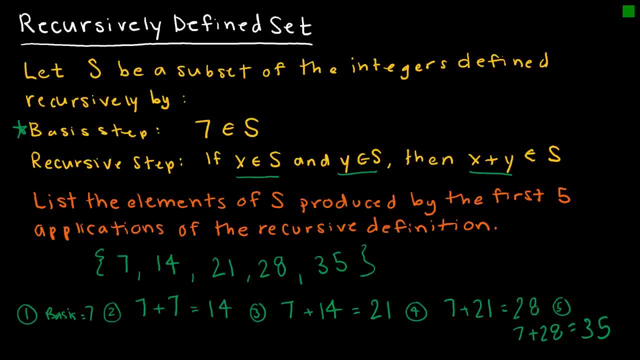 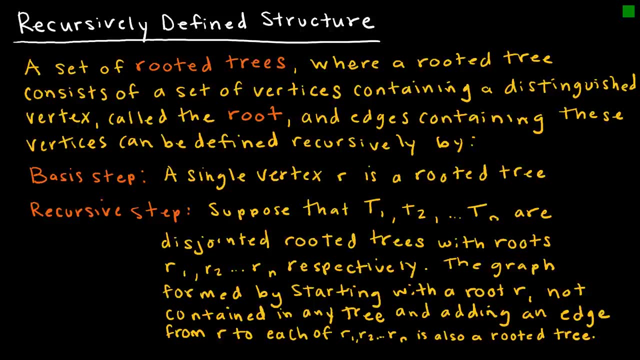 sum would also be in the set. I just wanted the first five, so I wanted to give you an example of a recursively defined structure rather than just a set. and I chose a rooted tree, because we're going to study rooted trees in an upcoming unit, and so I wanted to give you a good introduction. 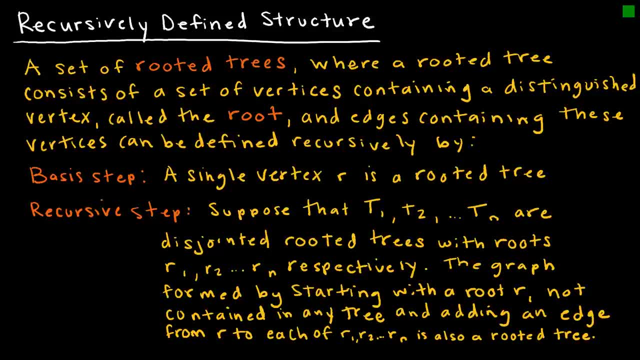 you can see that I have a set of trees and I have a set of trees and I have a set of trees, and so I wanted to give you a good introduction. so this says a set of rooted trees, where a rooted tree consists of a set of. 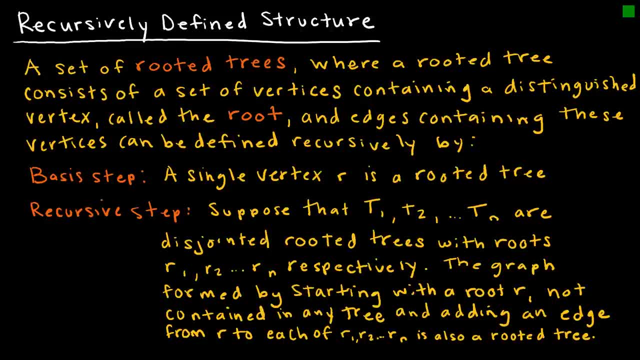 vertices containing a distinguished vertex called the root and edges containing these vertices can define, be defined recursively by the basis step. that says: I have a single vertex, so let's say here's my single vertex, R, that is a rooted tree. the recursive step says: suppose that you have tree 1, tree, 2 tree. 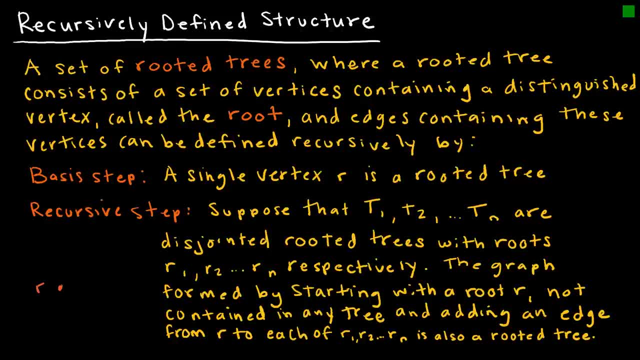 3, etc. all disjointed rooted trees. disjointed means are not connected to one another, but they're all rooted. trees with roots are one are two respectively. the graft form, by starting with a root R that's not contained in a tree and adding an edge from R to each of those roots, is also a rooted tree. so let's say I have a rooted. 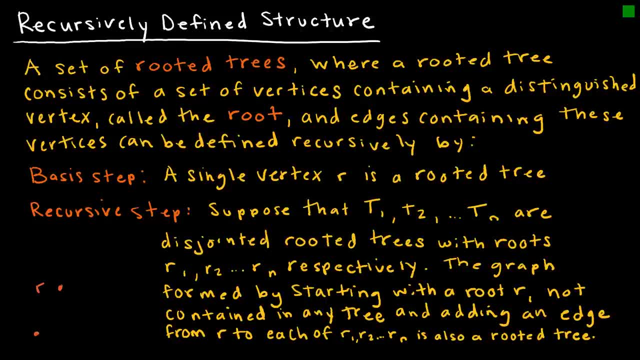 tree that looks like, we'll call that R. one that looks like this: so that's my rooted tree, we'll call that tree one. and the recursive step says: hey, if I take a new root that is not contained in any other tree and I connect it to the other roots, then I have a rooted tree. so I 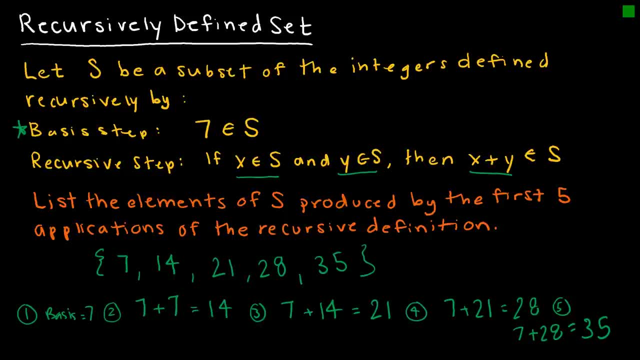 would in fact be what I would get if I took 42, which is what the next value would be plus 7.. So I can add two other elements of the set together and that sum would also be in the set. I just wanted the first five. 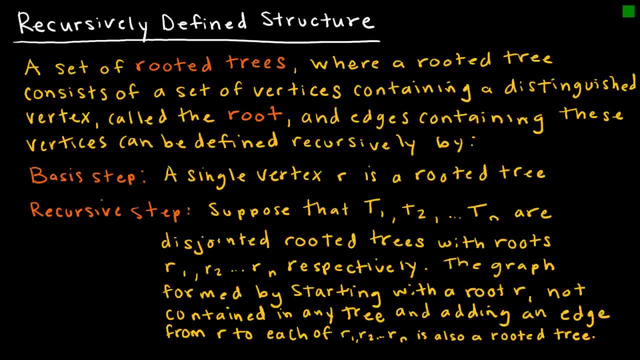 So I wanted to give you an example of a recursively defined structure rather than just a set, and I chose a rooted tree because we're going to study rooted trees in an upcoming unit and so I wanted to give you a good introduction. So this says a set of rooted trees, where a rooted tree consists of: 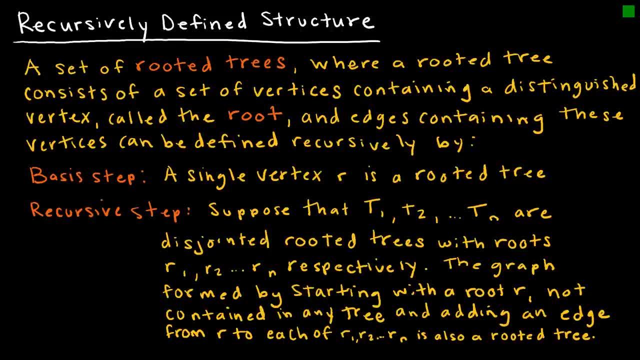 a set of vertices containing a distinguished vertex, called a set of vertices. The root and edges containing these vertices can be defined recursively by the basis step. that says I have a single vertex. So let's say, here's my single vertex R. that is a rooted tree. 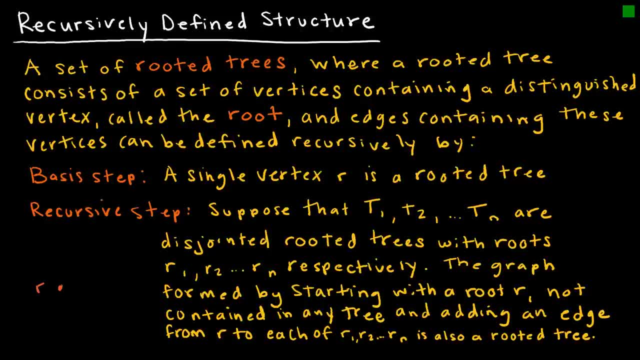 The recursive step says: suppose that you have tree 1, tree 2, tree 3, etc. all disjointed, rooted trees. Disjointed means they're not connected to one another, but they're all rooted trees with roots R. 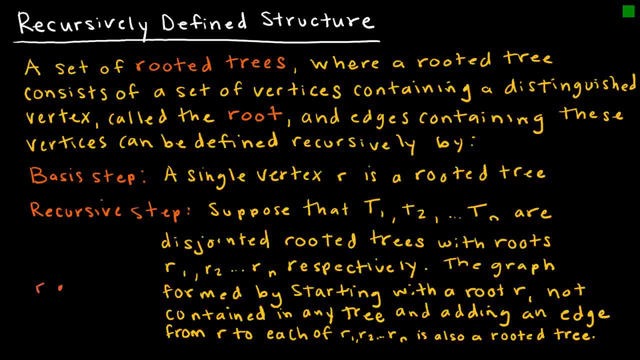 R1, R2, respectively. The graphed form by starting with a root R that's not contained in a tree and adding an edge from R to each of those roots is also a rooted tree. So let's say I have a rooted tree that looks like. 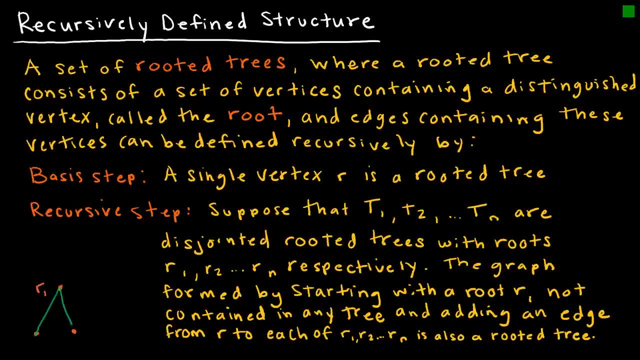 we'll call that R1, that looks like this: So that's my rooted tree. we'll call that tree 1.. And the recursive step says: hey, if I take a new root that is not contained in any other tree and I connect it to the other roots. 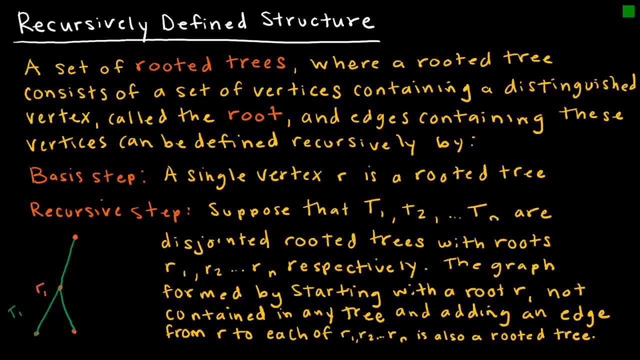 then I have a rooted tree, So I connected it to tree 1.. Well, let's say I also had a tree 2.. Well, if tree 2 looked like this, which is disjoint, then the recursive step says: take that R and that first. 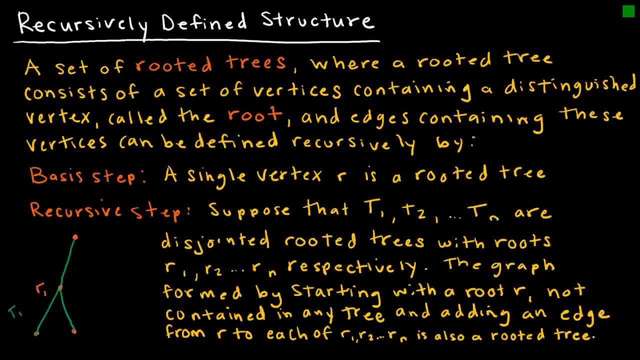 connected it to tree one. well, let's say I also had a tree too. well, if tree two is connected to the other roots, it looks like this: which is disjoint. then the recursive step says: take that R and that first, excuse me that first root that's not part of a tree, and connect it to those other trees and now all of a. 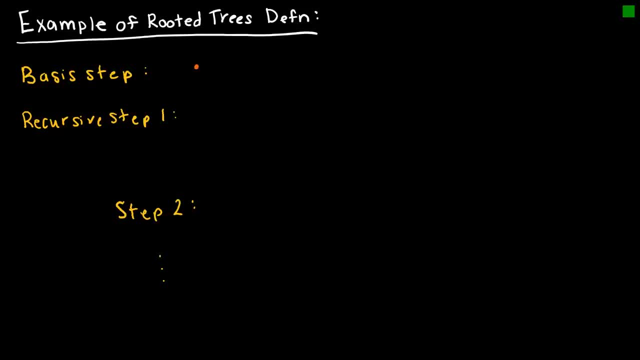 sudden you still have a rooted tree. obviously that's a little bit larger. so let's take a look at what that would look like using the recursive definition. this step again would just be one root. The recursive step says you can take that one root and add another root. You can take that one root and connect it to. 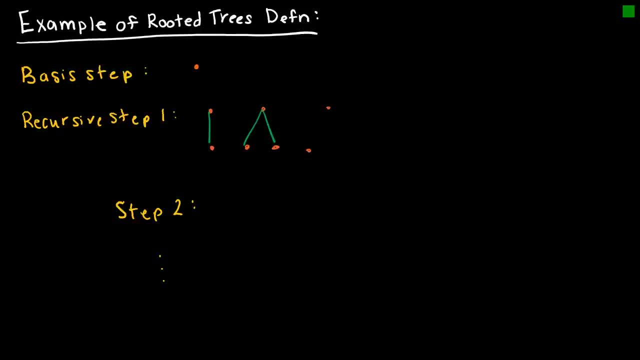 two others. You can take one root and connect it to three others and you get the idea I could continue. If I then applied the definition again, the recursive step of the definition again, it's saying: take these structures that we came up with, which again go on forever, and now repeat that step again. 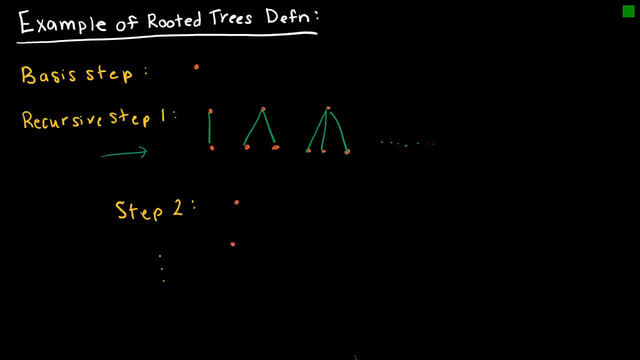 So if I had my original that looked just like this, that recursive algorithm says: hey, you can also just add one more if you want to. Or I could take my original that looks like this and say, okay, you can actually do two more off of that. Oops. 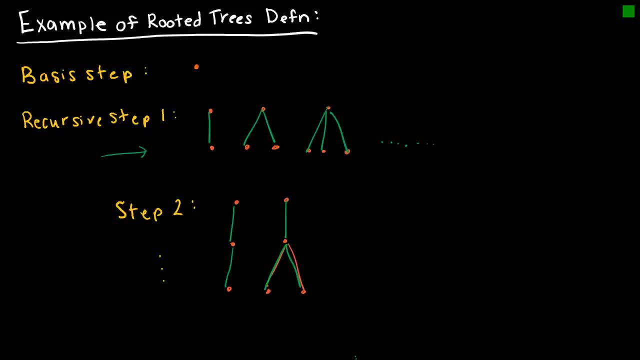 that's the wrong color. You can do two more off of that. Or I could have used this one and done the same thing, Or I could have used this one, Or I could have used one that I didn't even write down, And then, off of step three, I would be taking these structures and then adding essentially: 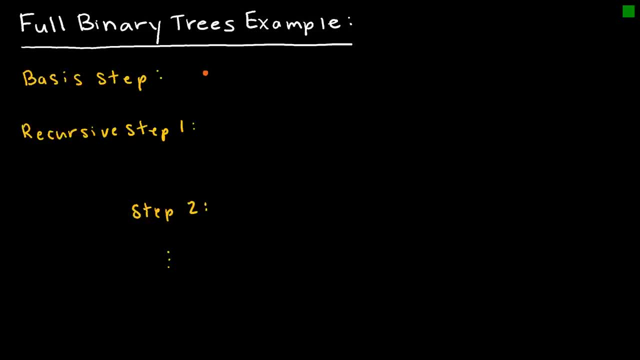 another row, another height. I didn't write the definition for a binary tree, but I did want to show you what a binary, a full binary tree is. And a full binary tree again has the basis step of just a root, The recursive step. one takes that root and connects it to two vertices Again. 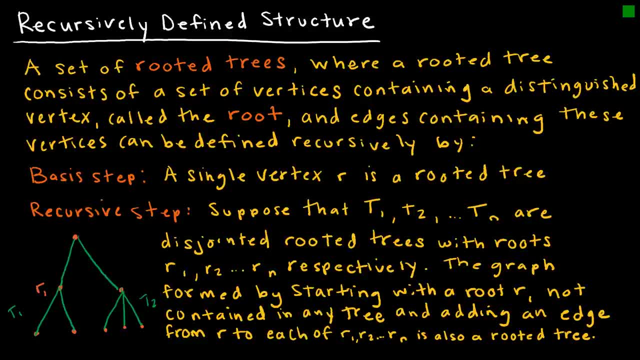 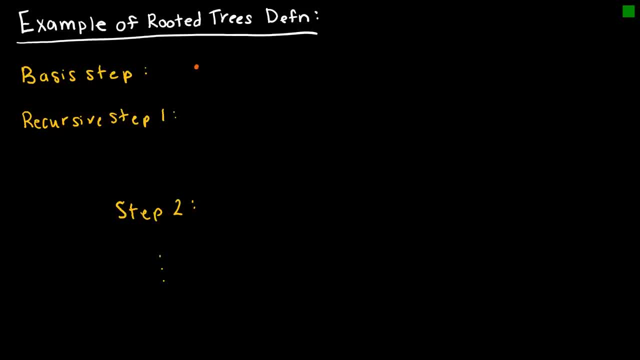 excuse me that first root that's not part of a tree and connect it to those other trees, And now, all of the sudden, you still have a rooted tree. Obviously, that's a little bit larger, So let's take a look at what that would look like using the recursive definition. 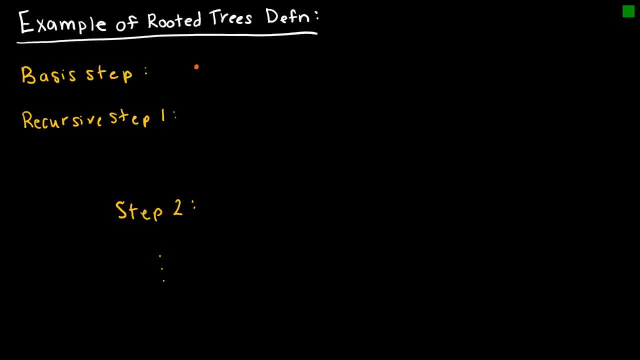 The basis step again would just be one root. The recursive step says you can take that one root and add another root. You can take that one root and connect it to two others. You can take one root and connect it to three others. 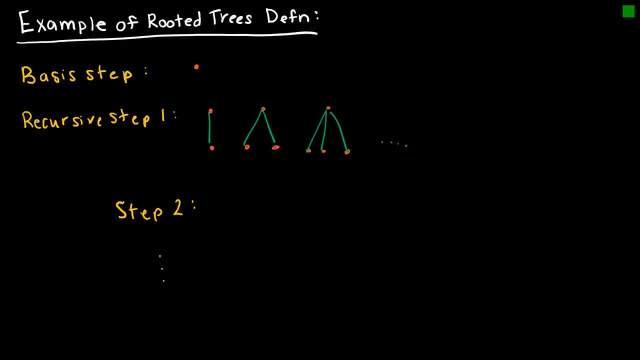 And you get the idea. I could continue If I then applied the definition again, the recursive step of the definition again. it's saying: take these structures that we came up with, which again go on forever, And now repeat that step again. 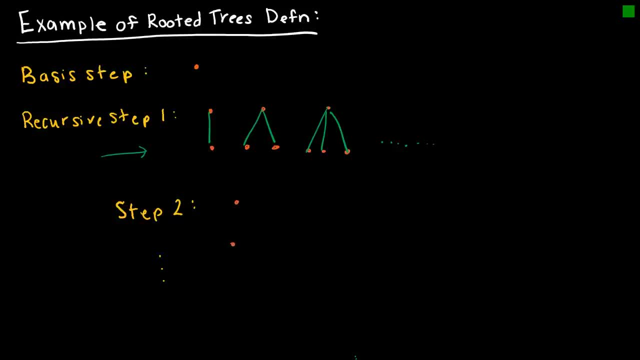 So if I had my original that looked just like this, that recursive algorithm says, hey, you can also just add one more if you want to. Or I could take my original that looks like this And say, OK, you can actually do two more off of that. 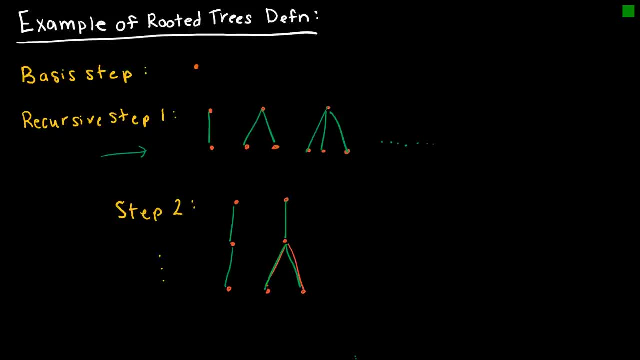 You can do two more off of that. I could have used this one and done the same thing, or I could have used this one, or I could have used one that I didn't even write down, And then, off of step three, I would be taking these: 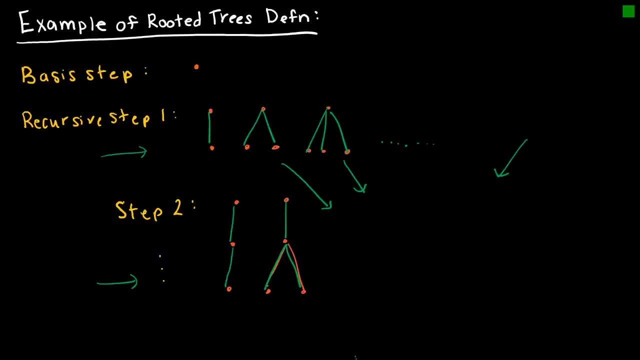 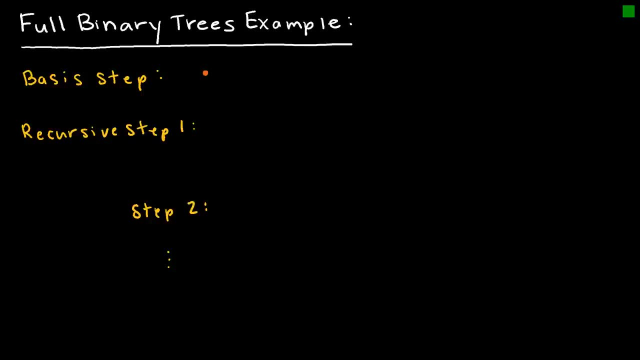 structures and then adding essentially another row, another height. I didn't write the definition for a binary tree, but I did want to show you what a binary, a full binary tree is. And a full binary tree again has the basis step of just a root, The recursive step. one takes that root and connects. 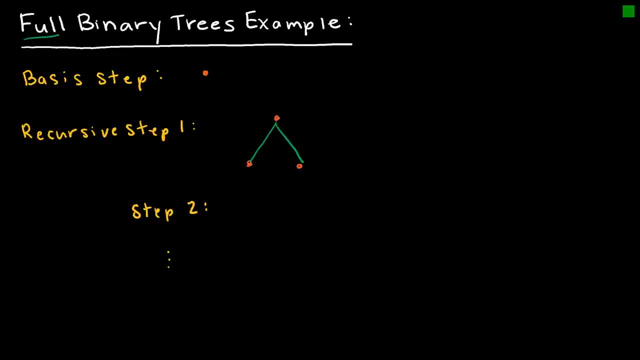 it to two vertices again, because this is a binary tree and binary implies two. Step two, and again there's no dot dot dot here because there's nothing else I can do. Step two says: take that initial structure, and I'm just going to draw it three times so I don't have to keep switching markers.